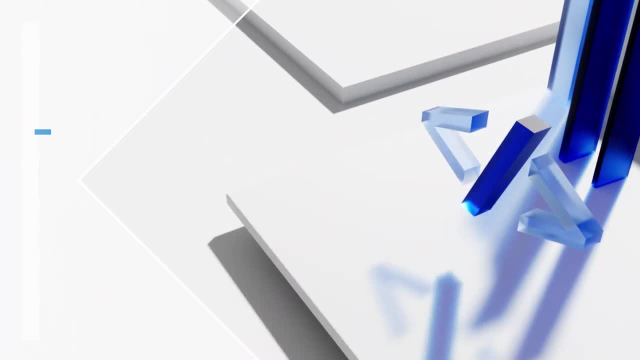 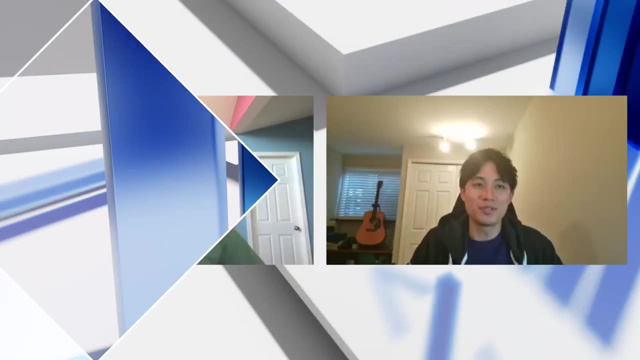 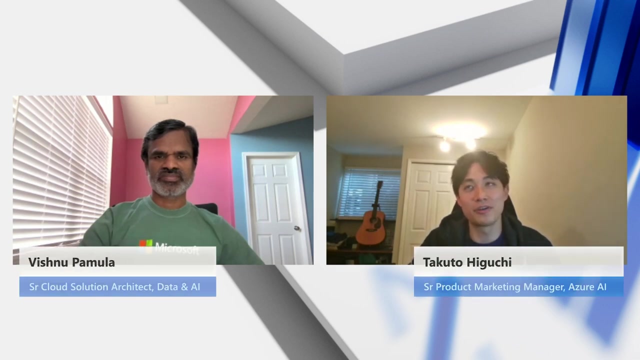 Welcome to our video series on LLM Ops, where we explore the journey of bringing generative AI applications into production. My name is Takeda Higuchi and I'm in the Azure AI product marketing team. With me today we have Vishnu from the Customer Success Unit team. 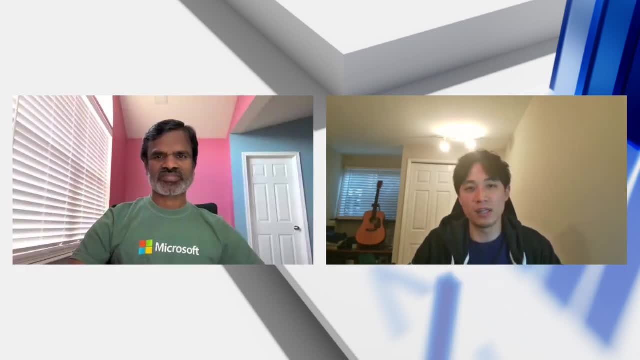 During the course of this video series, we'll delve into the concept of LLM Ops, what's so important in the era of Gen AI and how you can get started with LLM Ops using Azure AI. Now, without further ado, let's get right into the first episode. So, in this episode, 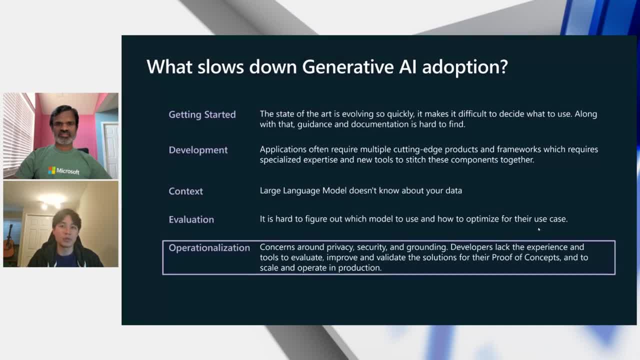 we'll focus on the introduction of LLM Ops as well as the first step of the journey, which is ideating and exploring. But let's start with why LLM Ops? As you know, Gen AI is everywhere today. But despite the promise of Gen AI, there are some challenges to fully. 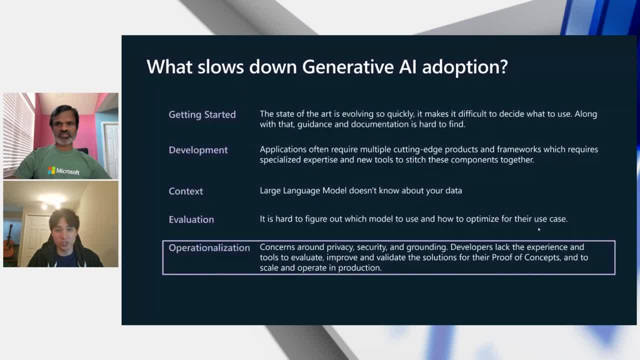 adopt and build your own generative AI applications. in production, Challenges include model accuracy, hallucination compliance, data privacy and security concerns. Additionally, integrating diverse data sources and absence of standardized lifecycle processes for model personalization and governance have been significant hurdles. 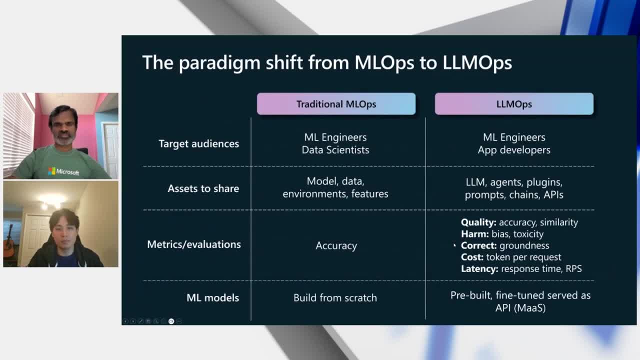 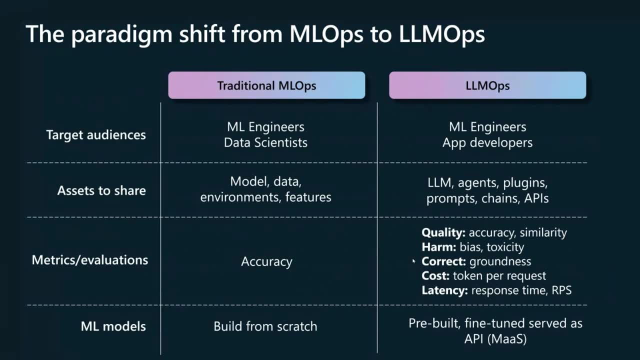 And we're witnessing a shift from traditional ML Ops to LLM Ops, tailoring these operational lifecycle to leverage large language models. LLM Ops focuses on enabling ML engineers and app developers with assets like LLMs, agents and APIs, and emphasizes metrics such as accuracy. 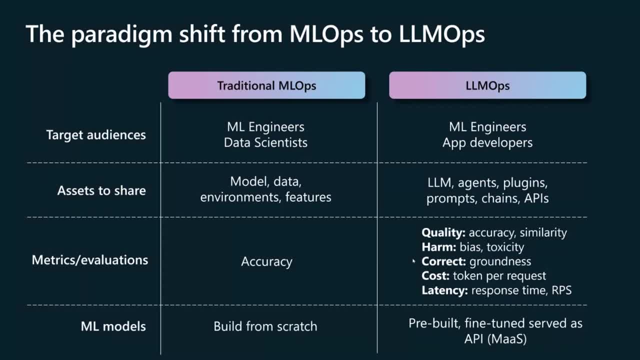 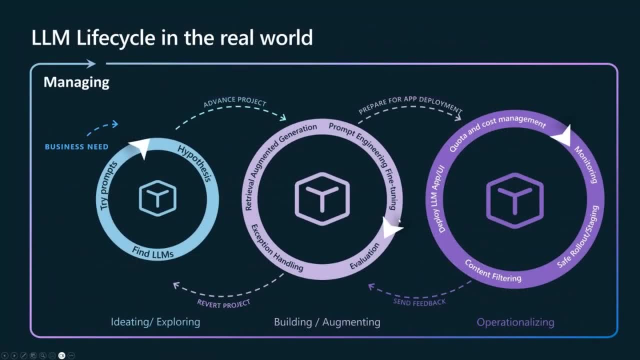 quality and cost. This shift is about enhancing efficiency and managing the unique demands of Gen AI In the real world. we believe that the LLM lifecycle looks like this: It includes three distinct loops, all encompassed by the fourth loop. The first one, ideating and exploring. 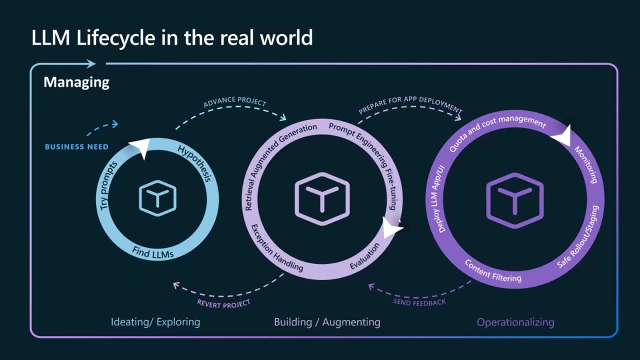 This is for finding and trying various LLMs, And the next one, building and augmenting. This is to augment the capabilities of LLMs with RUG and prompt engineering. And then third one, operationalizing. This is to actively monitor. 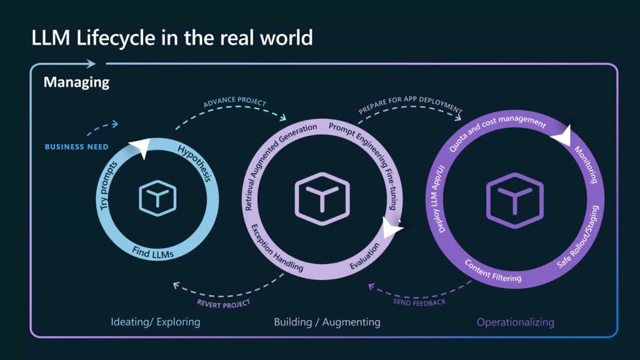 monitor models and apps and managing to make sure that everything is running in a compliant and insecure manner. So now you have a basic understanding of what LLM Ops is and how its lifecycle looks like. let's dive into the first loop, which is ideating and exploring in this episode. 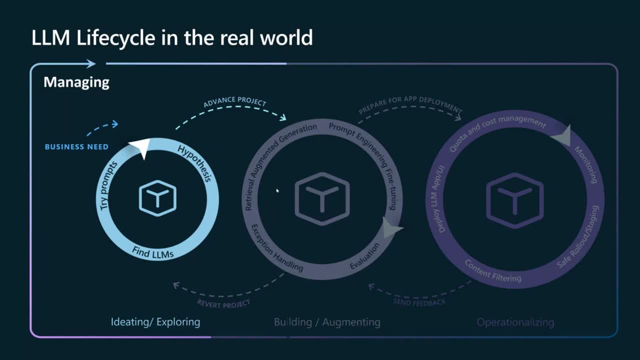 You learn how to discover LLMs in the Azure AI modal catalog, How to leverage model as a service, which allows you to deploy and fine tune models without managing any extra ergonomics underlying infrastructure. and how to use benchmarking to assess which model meets your. 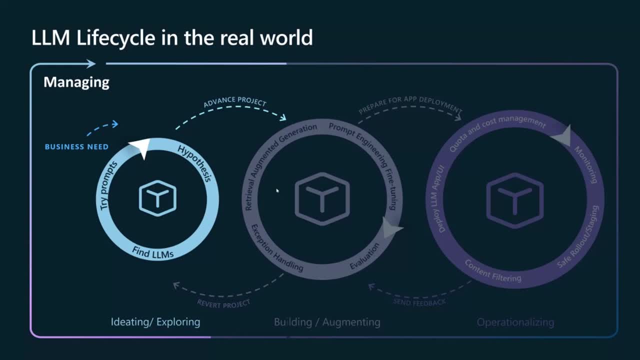 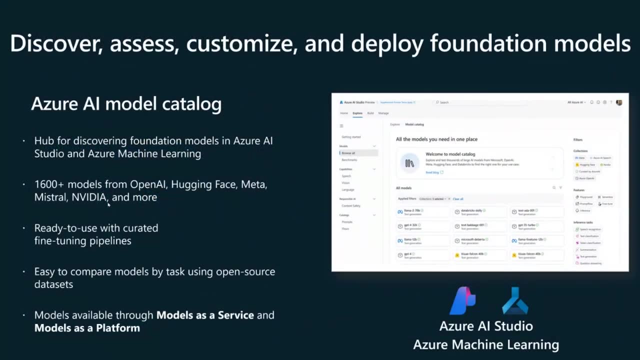 business needs and how to search prompt catalog with sample prompts. A key feature in this loop is Azure AI Model Catalog. available in both Azure AI Studio and Azure Machine Learning Model Catalog is a hub for discovering foundation models. The catalog includes some of the most 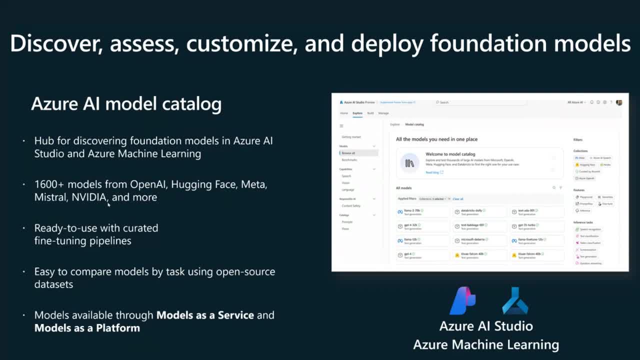 popular large language and multi-modal foundation models created by Microsoft: Hugging Face, Meta Mistral and also Azure OpenAI Service. These models are packaged for out-of-the-box usage and are optimized for use in Azure AI. At Ignite last year, we introduced the availability of 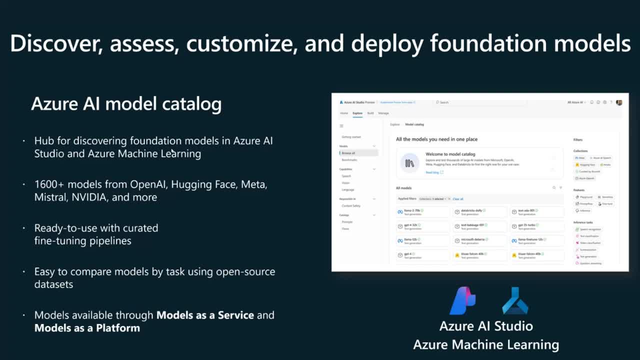 Model-as-a-Service that offers pay-as-you-go inference APIs and hosted fine-tuning, making it easier for developers to build GenAI apps by offering foundation models as an API without the hassle of managing deployment. The model is also available in MISTRAL's large model and MISTRAL's large model. We're actively 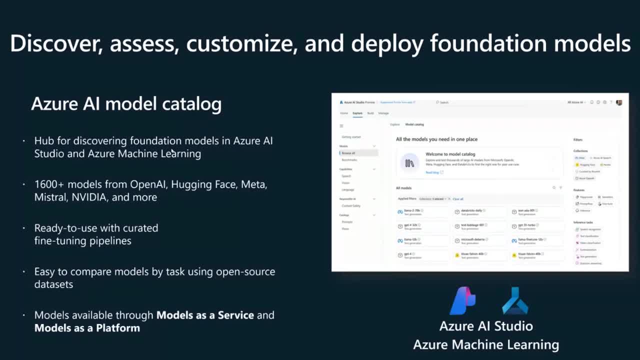 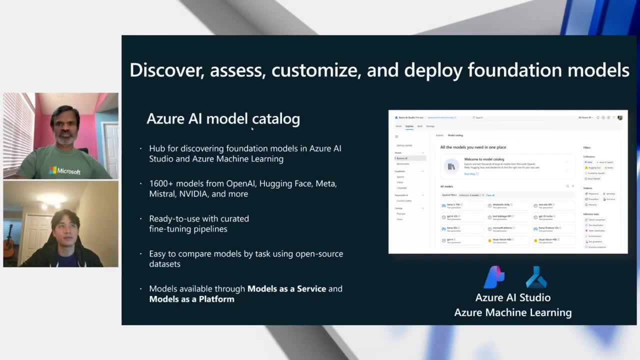 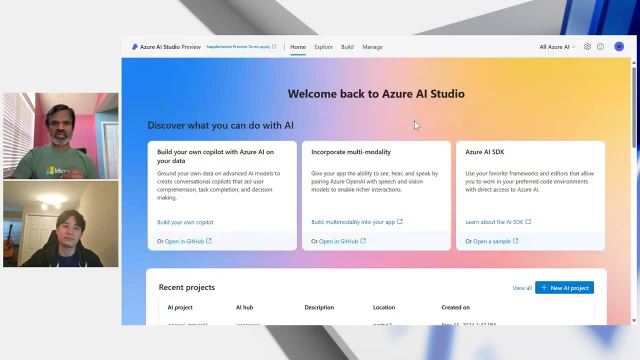 working with various model providers to bring their models to MAST. With that, I'm passing the button to Vishnu to see the ideating and exploring loop in action. Thank you, Takutu. In order to discover the models in Azure AI Studio, we have to 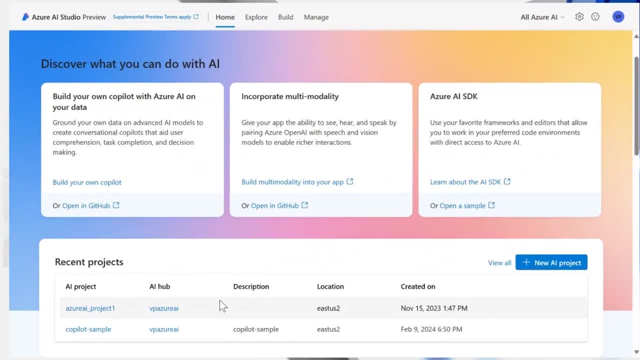 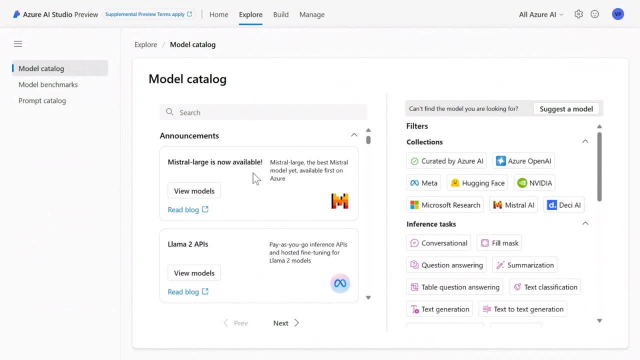 create a project first And then, once you have the project, you can go into the Explore tab, where we will see the recent announcements on the latest models, including MISTRAL, as you see there, And you will see all the models that Azure has created for you. We can 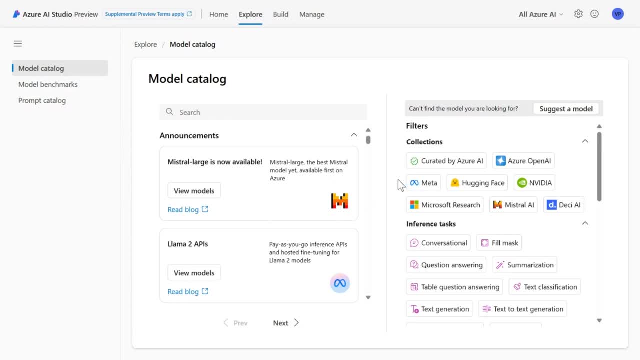 select the models by their model makers, for example, models from Meta by clicking on these collections- Hugging Face, OpenAI, MISTRAL and so on- And it's easy to also filter these models by the task itself, like if you are building a conversational or co-pilot, you can just select this. 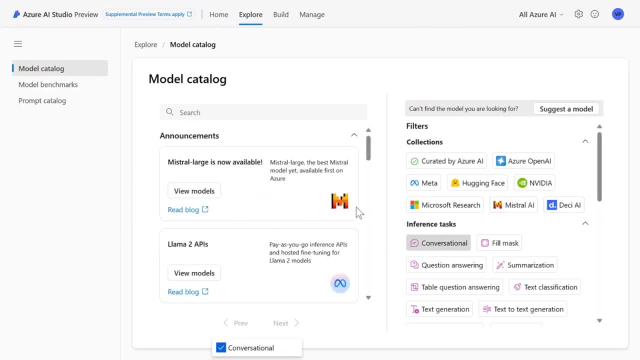 and it will show all those models. And, for example, if you want to deploy a Meta model like LAMA from Meta, you could select Meta and you will see all those models. If you want to deploy those models, you would click on, let's say, LAMA 27B And 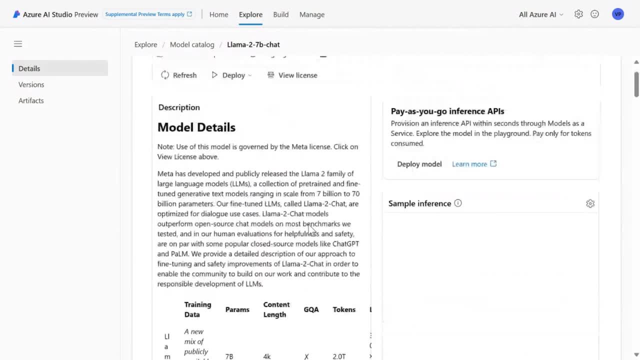 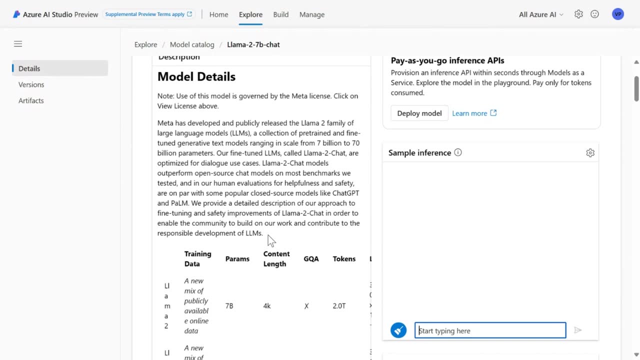 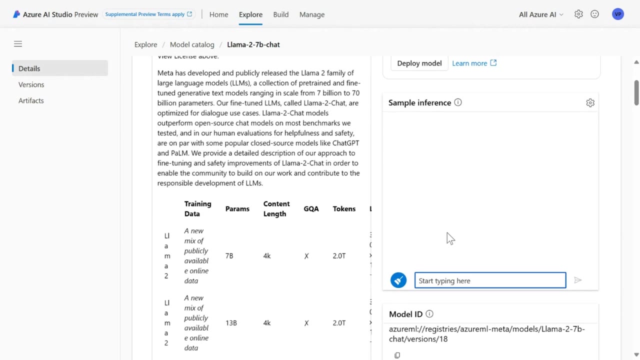 what Azure offers you is a nice interface here where you can see the model details and what this model is about, and you know the parameters it can take and so on. As Dakota was saying, without even deploying the model, you can use the model as a service. So 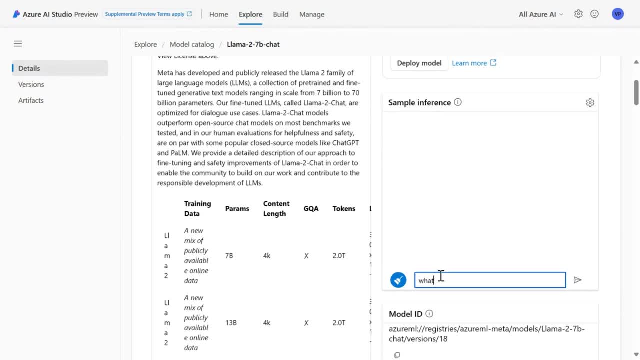 you can simply start asking questions here like what is, let's say, how far is a moon from the Earth? So you can start asking the questions right here, without even deploying the model. So see, right here you get the answers. If you want to deploy the model and you still have the option, you can also choose to deploy the model by clicking on the key here, So it can be used to deploy the models If you want to deploy the model and you still have the option. 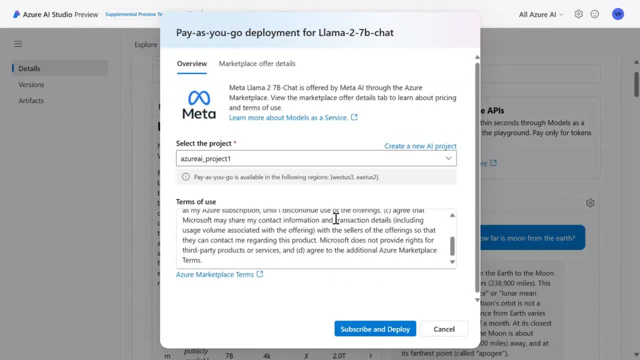 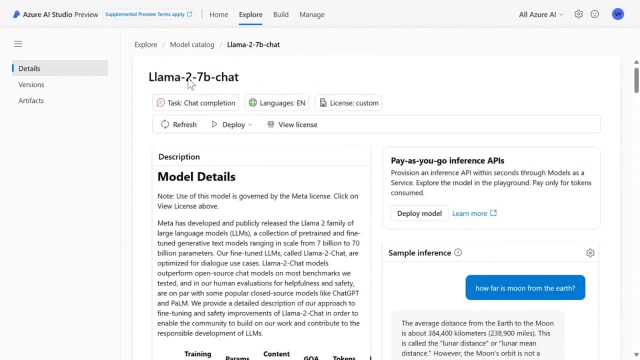 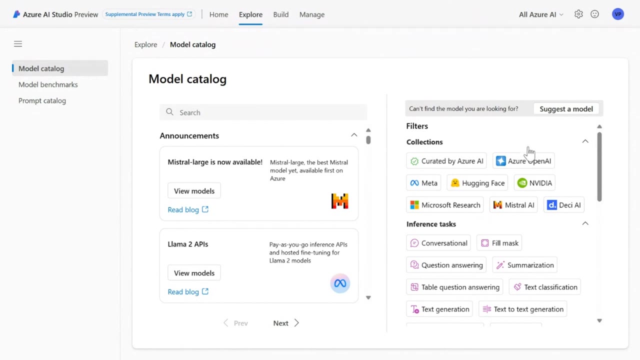 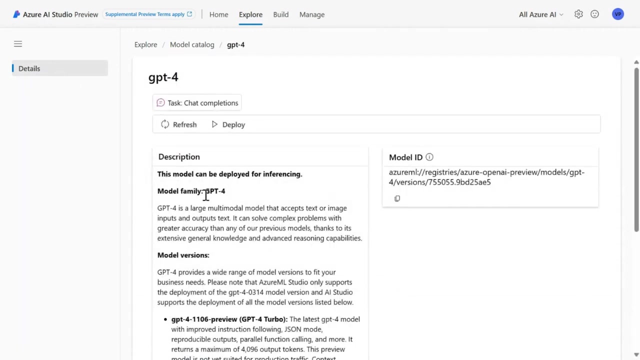 click on deploy and you can follow the instructions and with a click of a button model will be deployed. if you want to deploy the open AI models, it's slightly different because open AI models are already in Azure. so you would select the Azure open AI and let's say you want to deploy a GPT-4 model when